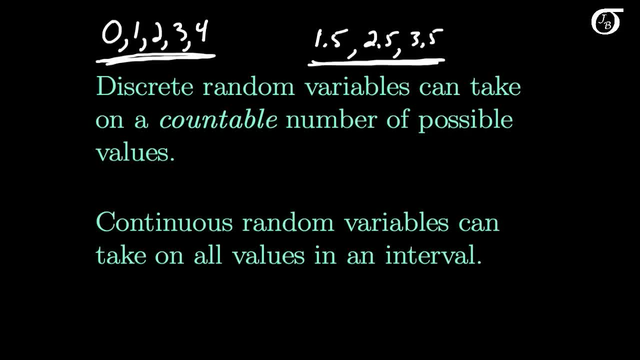 two liters And we went outside and put that in our backyard and we intended on coming out in a couple of weeks and seeing how much water was in there. Well, the amount of water in that container is going to be a random variable that can take on any value between 0 and 2.. 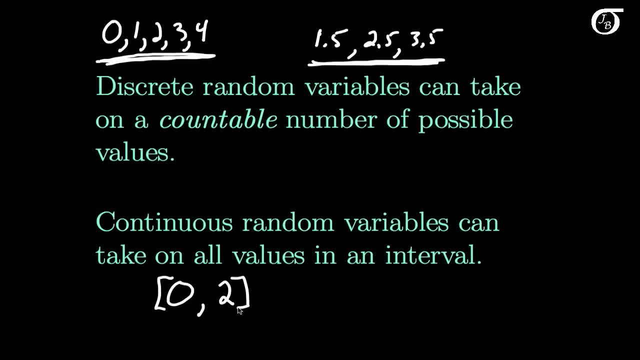 So any value in the interval 0 to 2 liters. But it can take on any value in there. So not just 0,, 1, and 2,, not just these distinct values like up here, anything in this interval. So an infinity of possible values in here. 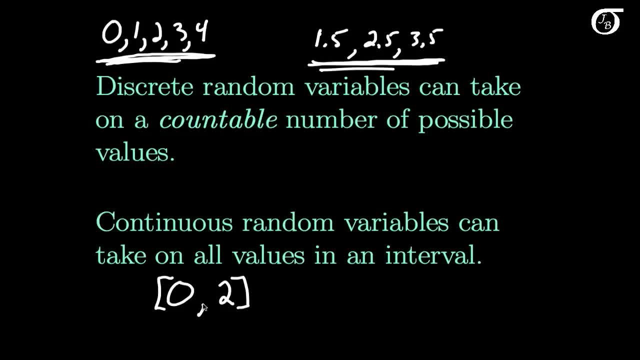 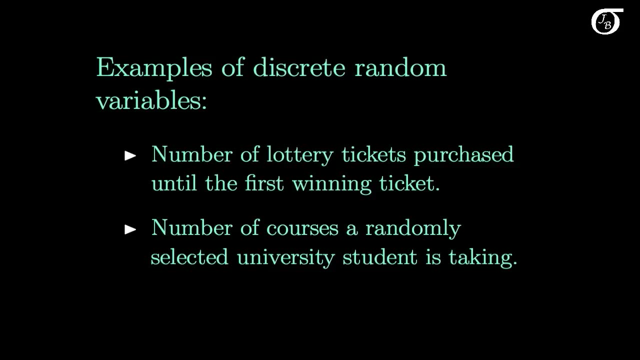 So 0, 0.3259862 liters, or any value between 0 and 2.. So there is a continuum there, an infinity of possible values between these two endpoints. Here's a couple of examples of discrete random variables: The number of lottery tickets purchased until the first winning ticket. 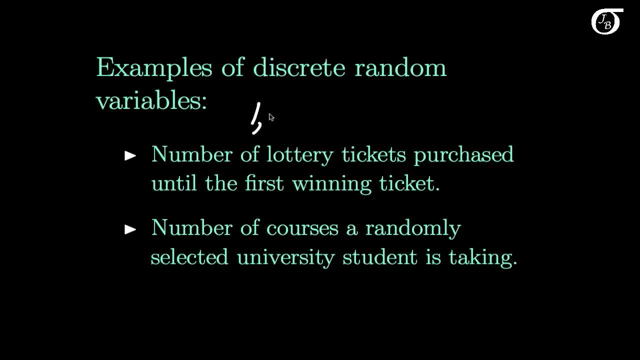 Well, we might get a winning ticket on our first ticket, or we might have to wait until our second ticket, or we might have to wait until our third ticket and there's no upper bound. so this is going off to infinity there. 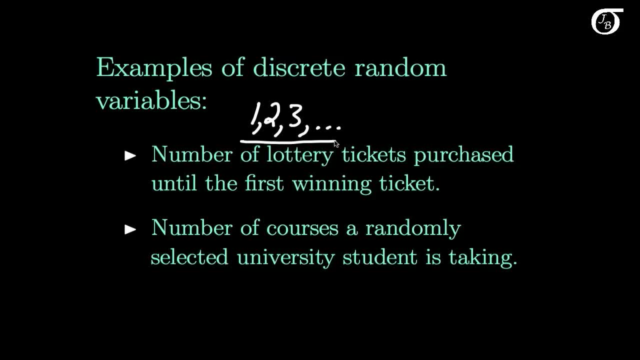 But even though this is going off to infinity, this is still a countable number of values. This is still a discrete, random variable. How about the number of courses a randomly selected university student is taking? Well, the possible values here are 0. 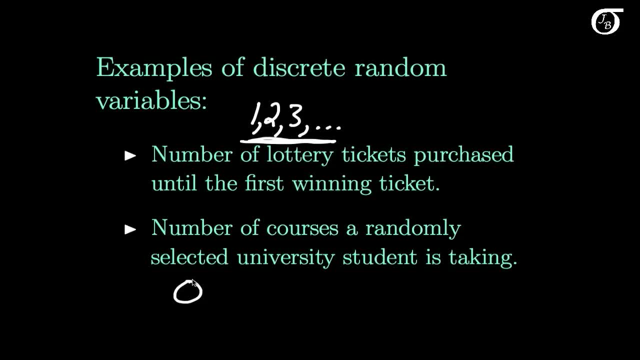 In some situations a person could still be considered a university student if they're taking 0 courses. for instance, some graduate students Or 0 or 1. Or 2, or 3, or There's some maximum here, but it depends on the university what that would be. 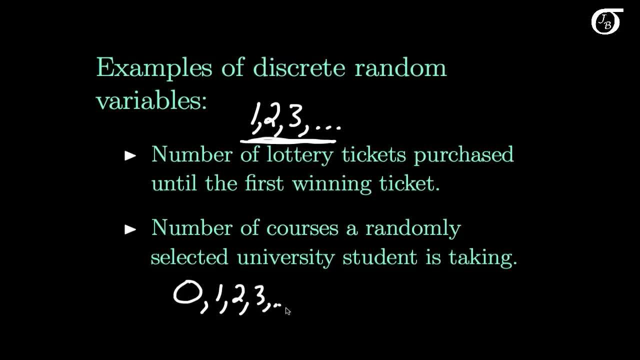 So there's some upper bound. maybe it's 5 or 6 or 7 or 8, but that would depend on the specific university. So that is still a countable number of values here, and so it is still a discrete, random variable. 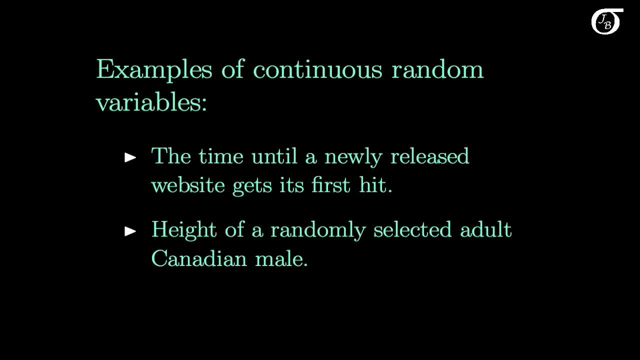 Here are a couple examples of continuous random variables. The time until a newly released website gets its first hit- Well, that's got to take on some value greater than 0,, right, So let's just say greater than 0.. And the height of a randomly selected adult Canadian male. 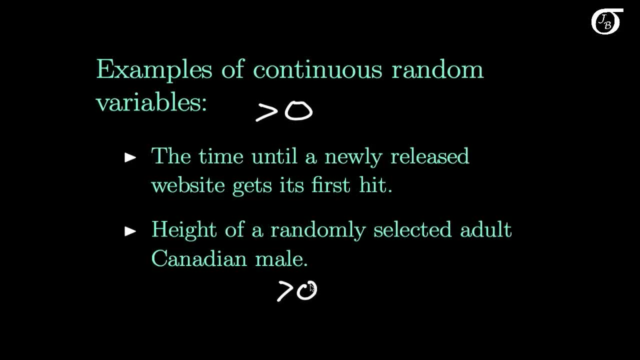 again, that's just going to take on some value greater than 0.. There is some minimum value. we don't have an adult Canadian male that's less than 2 centimeters tall, say, but there's no natural lower bound here, no natural upper bound. 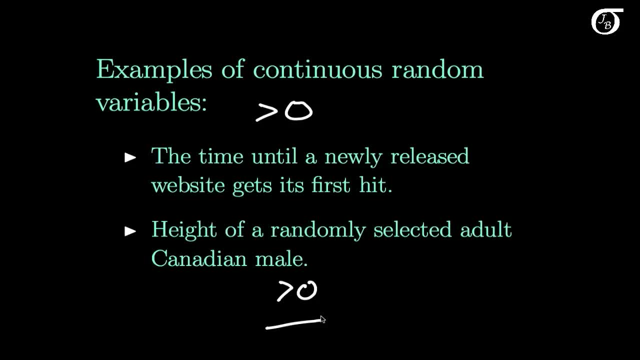 so let's just say some value greater than 0, even though in practical cases there's some more practical range of values. In either one of these cases there aren't discrete jumps. It's not like a person is 174 centimeters tall and then the next possibility is 175 centimeters tall. 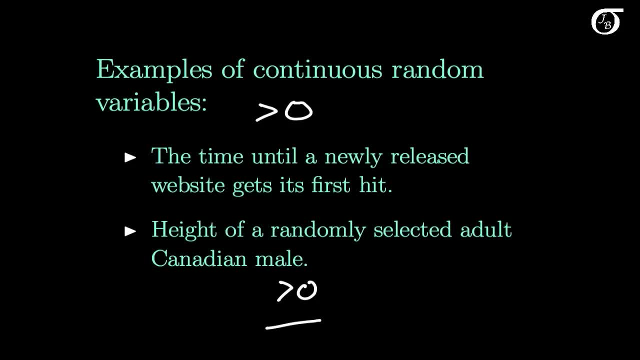 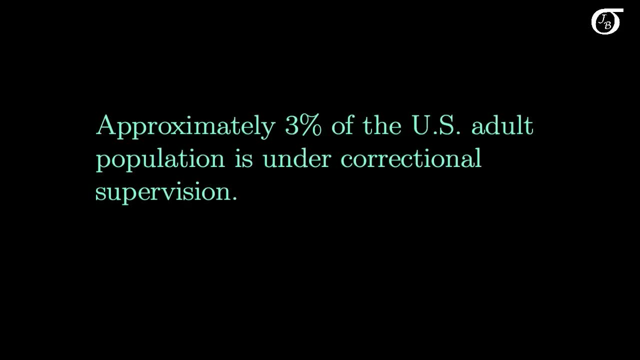 Anything in there. there's an infinity of values between those two possibilities, So these are continuous random variables. Let's go back to discrete random variables and look at an example. Approximately 3% of the United States adult population is under correctional supervision. 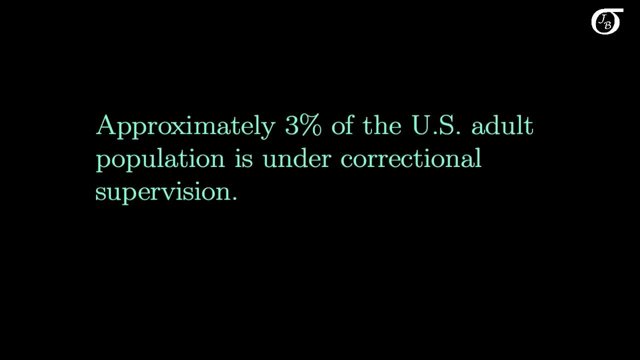 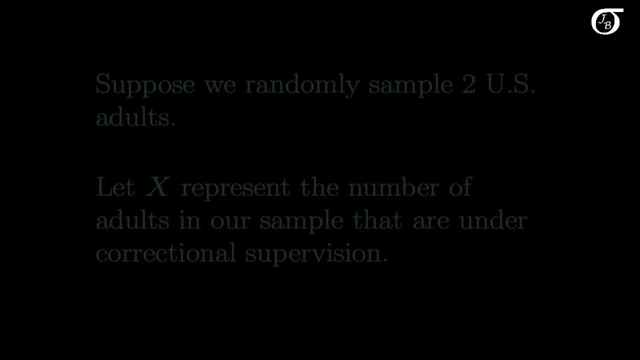 meaning they're either in jail or on probation or on parole. Now this 3% is approximately true, but let's pretend that's exactly true for the purposes of this example. Suppose we randomly sample two US adults and we let capital X represent the number of adults in our sample. 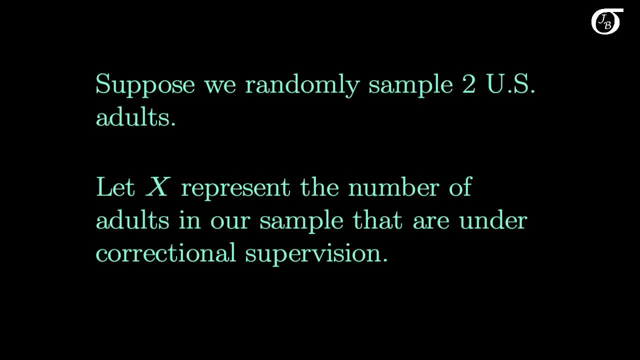 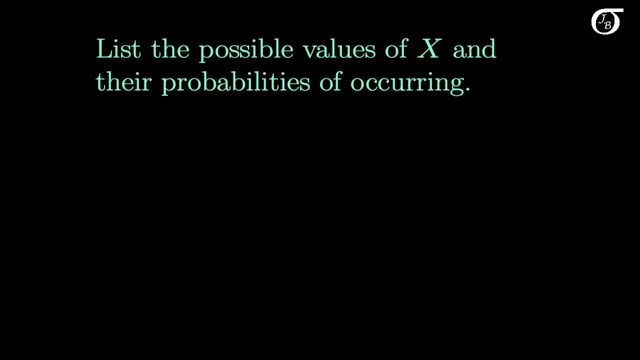 that are under correctional supervision. We typically represent random variables with capital letters near the end of the Roman alphabet, so very often we have X or possibly Y or possibly Z. Let's list the possible values of X and their probabilities of occurring. Well, the possible outcomes. 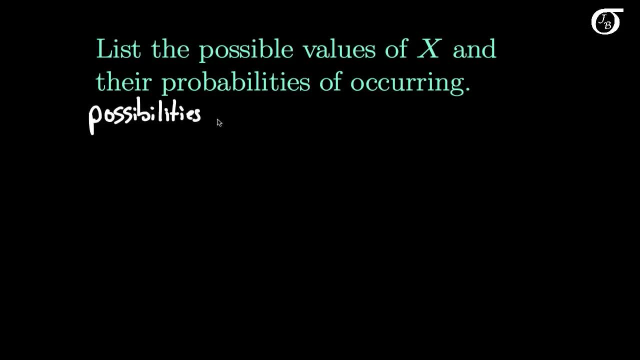 so, which I'm just going to label here, as the possibilities are that the first person we get is not under correctional supervision- that's one possibility, and the second person is not under correctional supervision as well. So I'm going to let N represent someone who is not under correctional supervision. 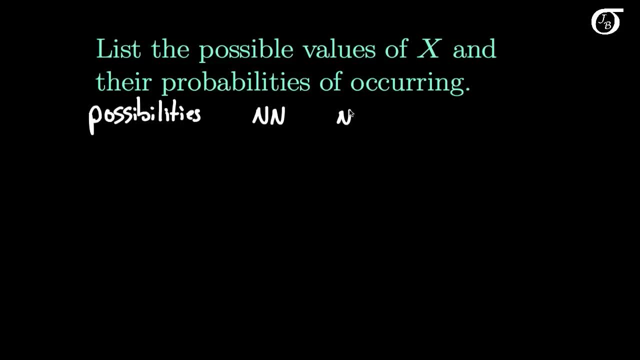 Another possibility is that the first person we get is not under correctional supervision, but the second person we get is under correctional supervision. Another possibility, of course, is that the first person we get is under correctional supervision and the second is not. 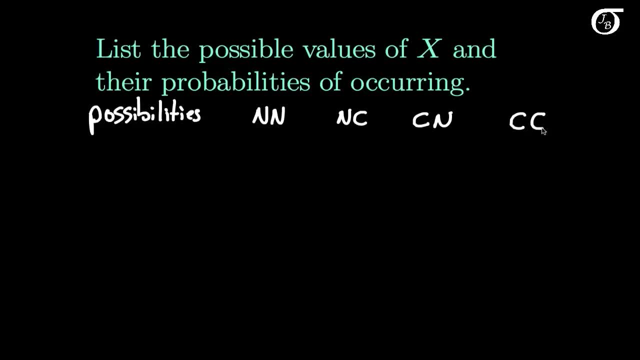 and the fourth possibility is that both people that we randomly sample are under correctional supervision. Now, the value of X, the value a random variable takes on in these spots. well, if you recall, X was the number of people that are under correctional supervision. 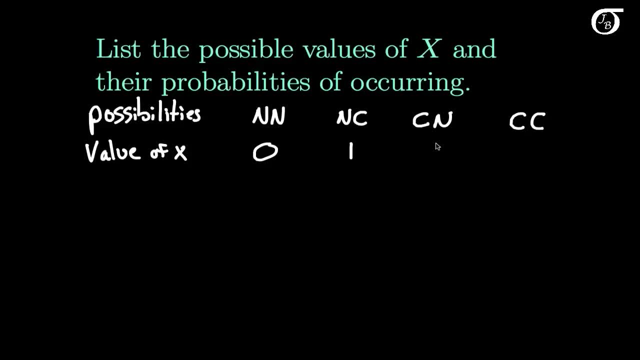 So here it takes on the value 0,, here it would take on the value 1,, here it would take on the value 1, and here it would take on the value 2.. Now let's list the probabilities here. So if we calculated the probabilities of these things happening, 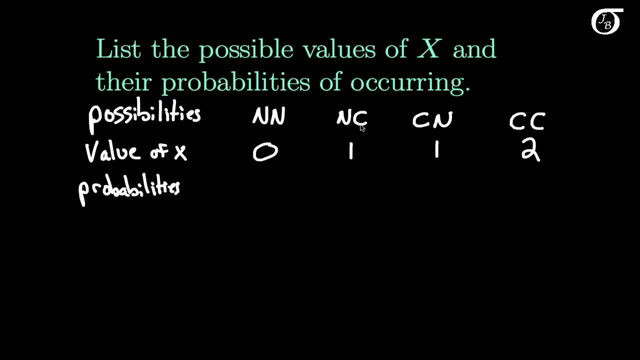 if we are sampling randomly and independently and the probability that a person is under correctional supervision is 3%, the probability they're not is 97%, And if they're randomly and independently, we can simply multiply those probabilities together here. So the probability of getting N and then N is 0.97 times 0.97. 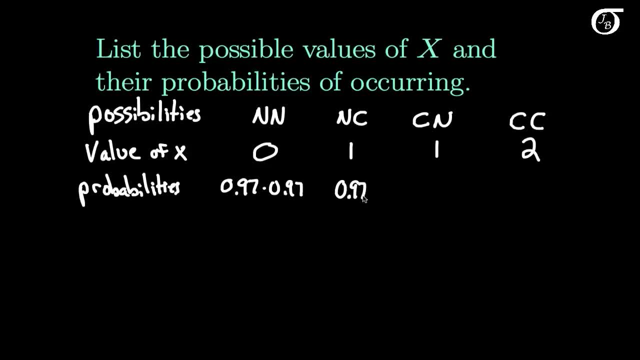 The probability of getting N and then N is 0.97 times 0.97.. The probability of getting C and then C is 0.97 and then times 0.03.. The probability of getting C and then N is 0.03 times 0.97. 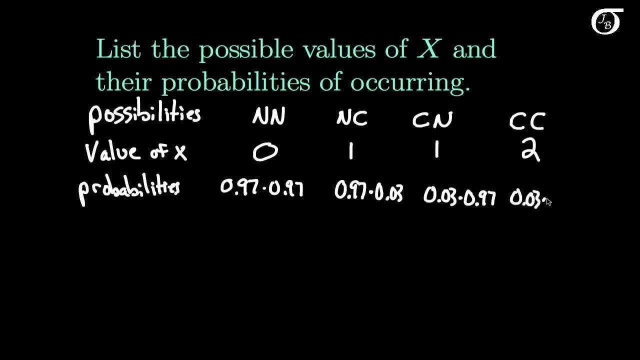 And the probability of getting two C's is 0.03 times 0.03.. Now this works out to 0.9409.. This works out to 0.0291.. Of course, this is the same thing: 0.049.. 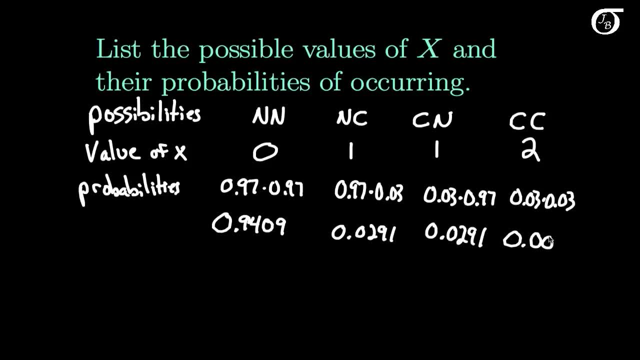 And this works out to 0.0009.. Now if we were to summarize that, if I said the value of X, if I summarize this with my value of X and said it can take on the possible values 0,, 1, and 2,, 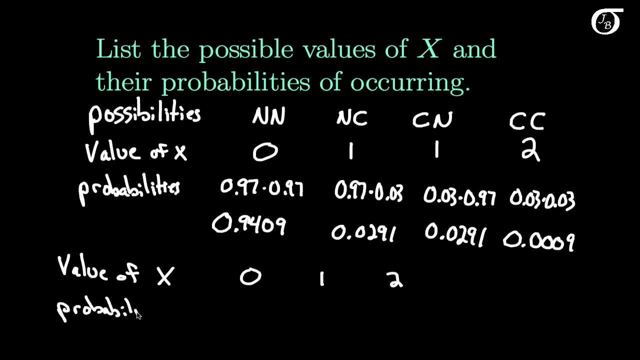 and the probability of those occurrences. of our random variable X, well, this one has a probability of 0.9409.. This one has a probability. well, one happens in these two spots. so this is going to be these two added up together. 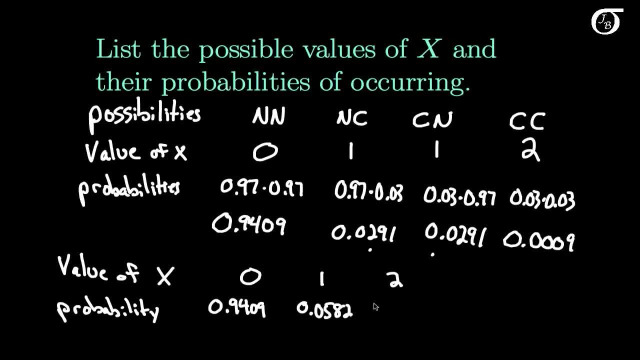 and we get 0.0582.. And 2 is 0.0009.. So we might say something like the probability that the random variable X takes on the value 2 is equal to 0.0009.. But we might want to just do this in general. 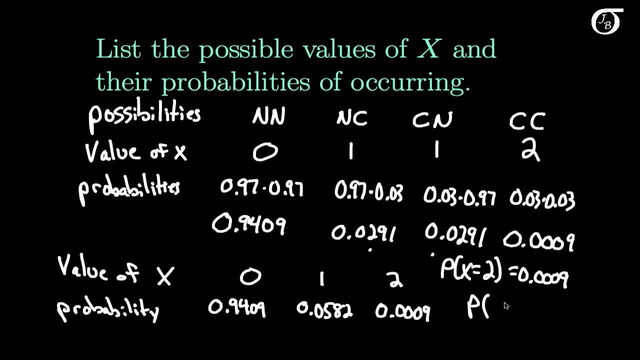 So we do want to write this sometimes. the probability that the random variable X takes on the value 2 is equal to 0.0009.. The probability that the random variable X takes on some value- And we call that some value, little x. 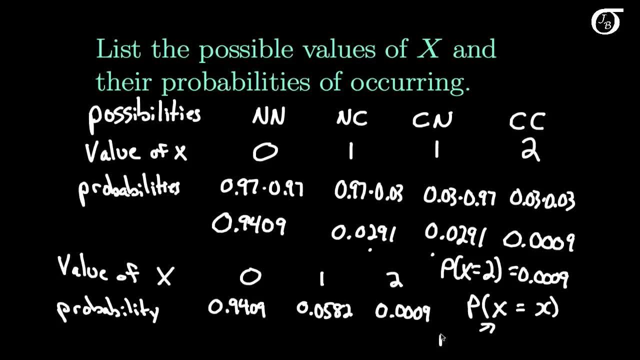 And the capital X represents the random variable X, whereas little x represents some value of the random variable X, So we could call this value of X. we could sometimes write that, as I'm going to put it in brackets here, little x. 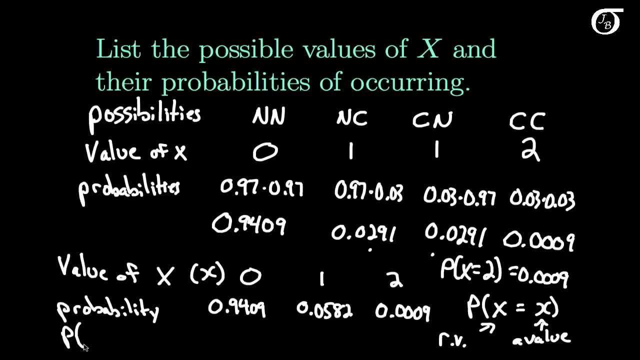 And this probability we represent as the probability that your random variable X takes on the value little x, And we sometimes write that as P. Now what we have here, what we have just done here, is created the probability distribution of our random variable X. 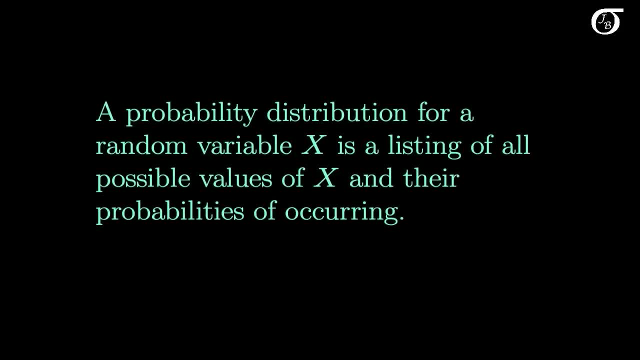 A probability distribution for a random variable. X is a listing of all possible values of X and their probabilities of occurring. Now, this can be a listing, like we had on the previous slide, or this can be a formula, or this can be some sort of graphic representation. 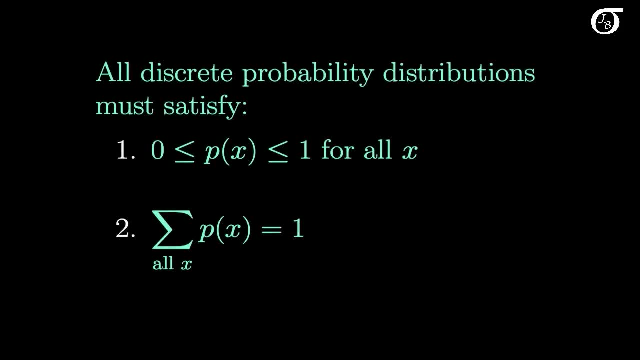 We know that all discrete probability distributions must satisfy these conditions. Little p represents a probability, and probabilities have to lie between 0 and 1.. So P is between 0 and 1 for all X, And we are listing all possible values of X and their probabilities of occurring. 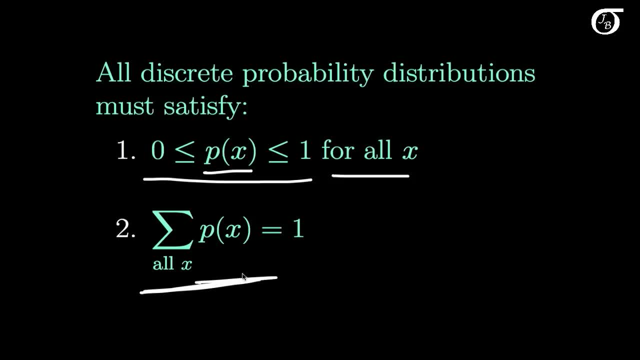 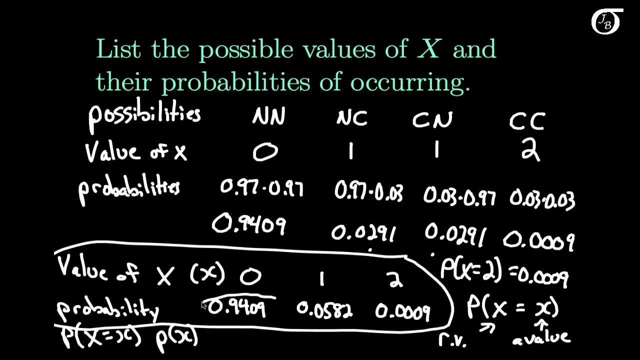 So if we sum up the probabilities of all possible values of X, we're going to have to get 1.. And if we go back to our discrete probability distribution here, we would see that the probabilities do in fact all lie between 0 and 1.. 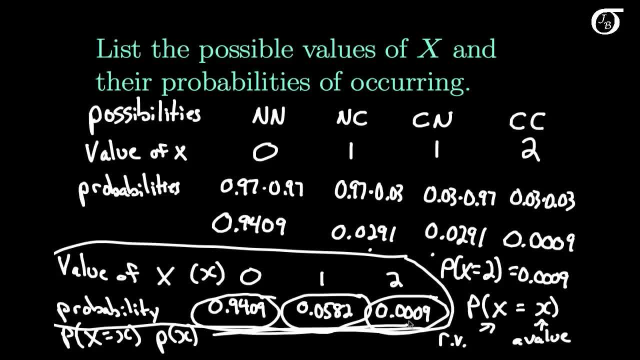 And if we added them up, we would see that they sum to 1.. Depending on the discrete probability distribution, these values can be anything. Here we have 2, that doesn't lie between 0 and 1.. Maybe it's negative, maybe it's a billion, depending on the situation. 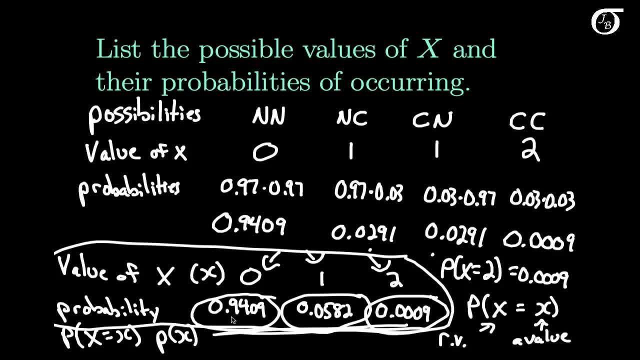 The values of X can be anything depending on the situation, But the probabilities have to satisfy those conditions on the previous slide. Now, we very often plot this out to see what this looks like visually. So let's plot these values of X and their probability of occurring.